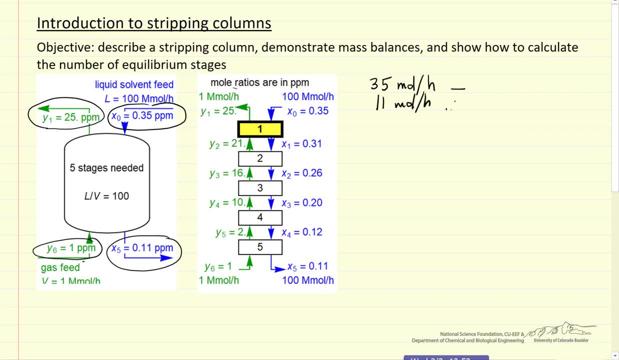 of 11 mol per hour in the liquid phase. so that says we've removed 24 mol per hour. If we look at the gas phase, we go from 1 ppm to 25 molar flow rate times the mole fraction. Indeed, we have a steady-state mass balance. We have now added 24 mol per hour to the vapor. 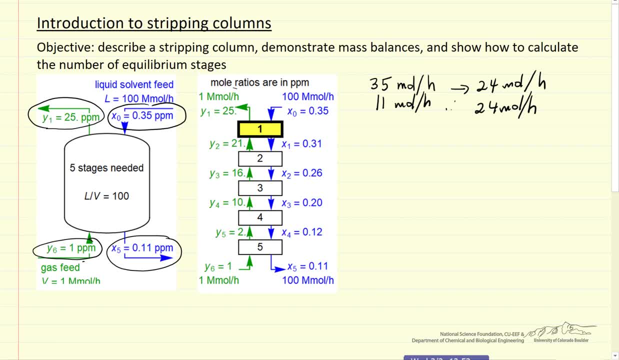 phase And you can see in this five-stage example, the mole fraction increases and the vapor actually increases in each stage. So one of the important numbers in the calculations you're going to do is the liquid to the vapor flow rate, and for this case it's 100 over. 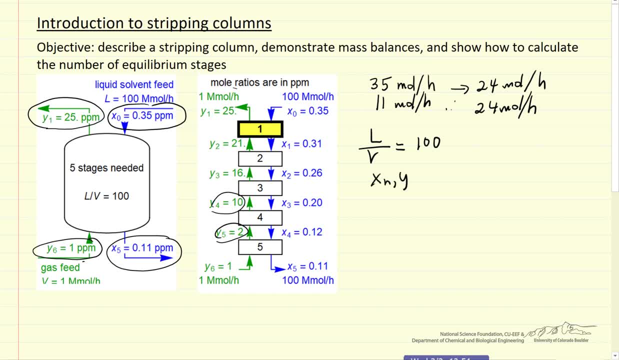 1. And other important thing to keep in mind is our notation xn, yn. These are two compositions, two phases of equilibrium. In other words, if I write x3 and y3, that means leaving stage 3.. The liquid mole fraction is xn. The vapor mole fraction, or mole ratio, is yn. Those 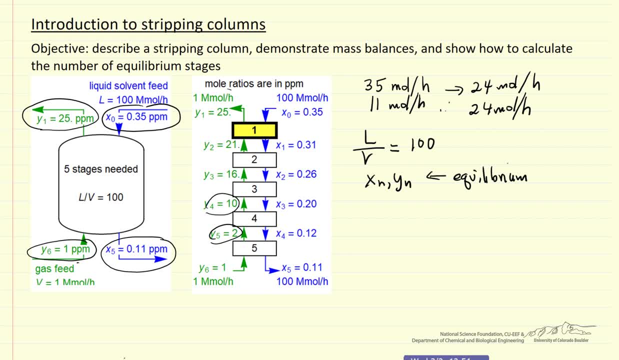 two are in equilibrium. Now the equilibrium we're modeling by a Henry's law because of low concentration. So Henry's constant over pressure times xn. So in this case Henry's constant has units of pressure. So what I'm going to do is pick three stages and I'm 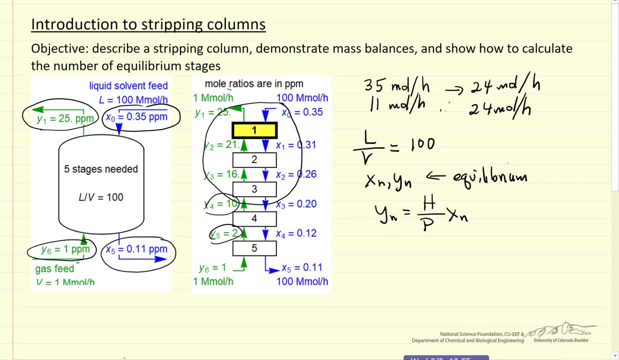 going to do a mass balance around here, And what that means is, if I look at what's going in for the solute, it should equal what's going out. So what's coming in is x0 times liquid flow rate, plus in the stage 3, is y4 times the vapor flow rate. What's leaving? 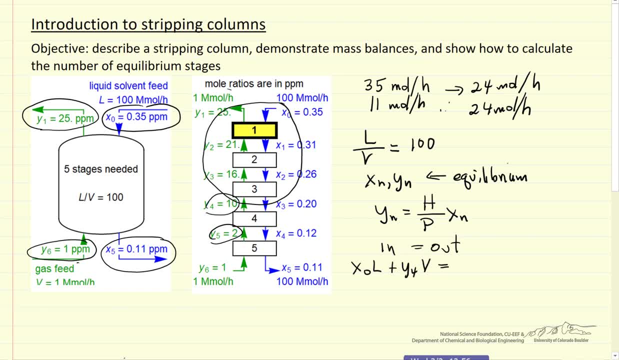 then is x3 times the liquid flow rate, times y1 times the vapor flow rate. Well, in, stop clear itCP. Do a ک, a plus 1.. This is xn times l, y1 times v. This forms the operating line, So let me rewrite it in terms. 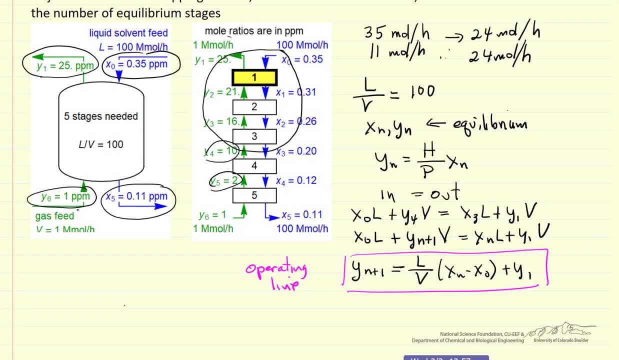 of y versus x. So to determine number of stages, I'm going to use a plot of y versus x. This is the operating line on that same plot. This, then, will be the equilibrium line. So let's look at a plot and put some numbers in, just to give you an idea how to determine the number of stages.